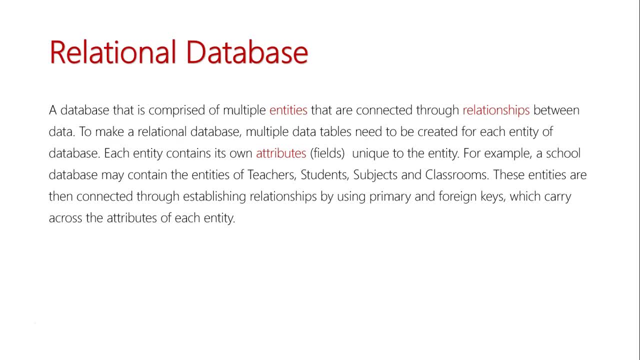 the details about each database. So basically what that means is, in the area of students, you'd have student name, their age, their parents' details, their email address, and then, under the entity of teachers, you'd have their teacher's name, what subjects they teach. 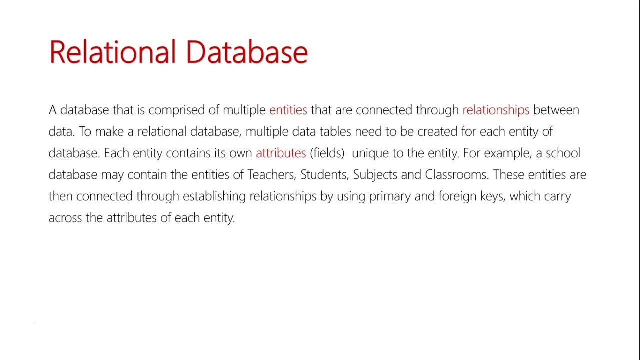 and so on. So they would be the attributes for each of these separate entities. Now, there'll be times where we need to do that To connect all these entities together, such as creating the school timetable. This is done through establishing relationships. Now, this is where the power of a relational database 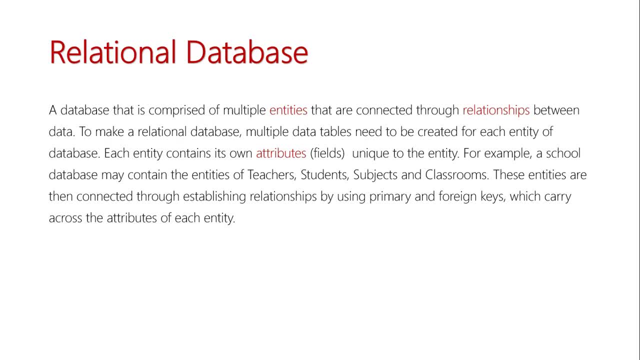 is because we can pull all that data across by bringing across just the primary key and by making it a foreign key, it allows us to connect all the attributes in one table to another. Okay, so let's take a look at how we can do this in Microsoft Access. 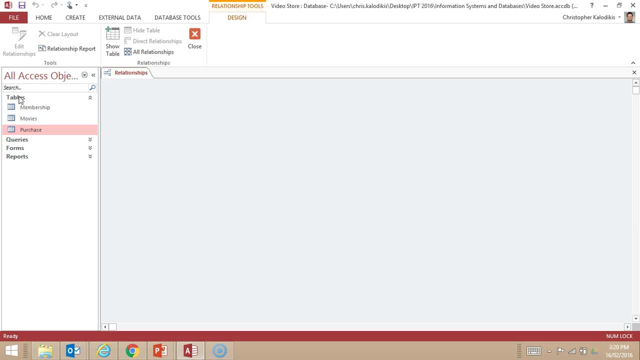 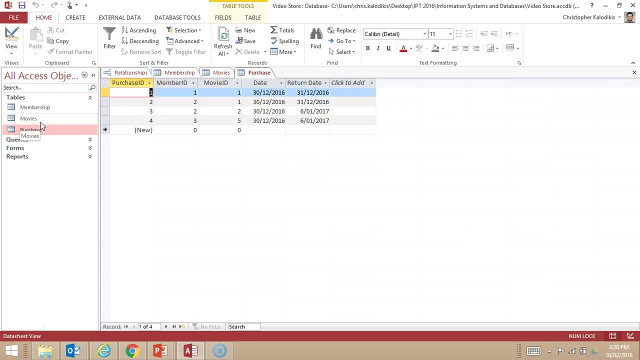 So here you can see, on my left, I've created three tables: membership, movies and purchase. Now these could be for some sort of movie rental system. Okay, so I've established these three different tables. Now, if you take a look at these tables, membership has its own. 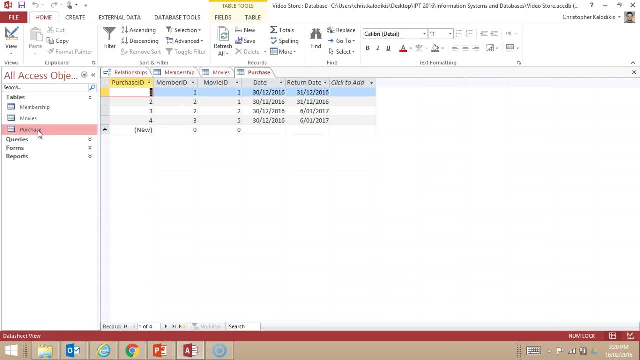 ID field. movies has its own ID field, And then in the purchase table I can see that the membership ID and the movie ID are also here as well. Okay, By these two existing here they are known as foreign keys and they are my reference. 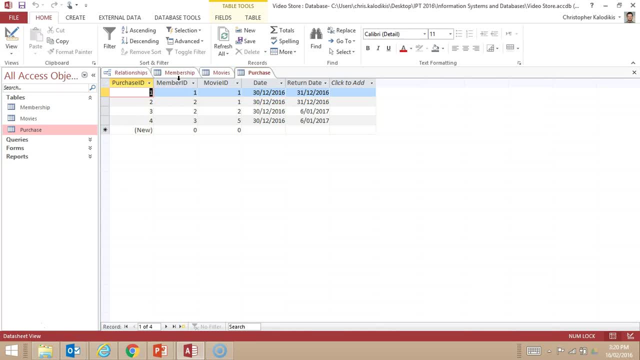 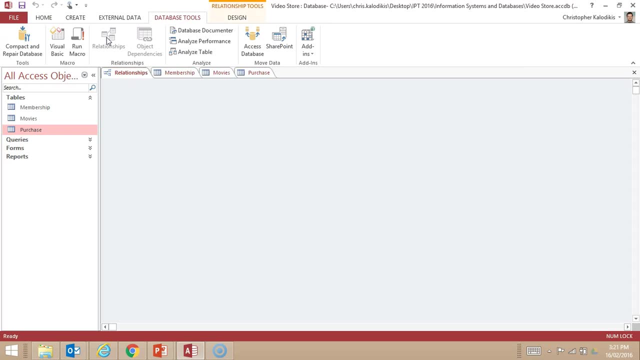 point back to the other two entities. Okay, so now I'm going to make my relational database now. So, in order to do that, I'm going to go to database tools and I'm going to go relationships. I'm going to close my database tables so I don't get any problems, Okay. 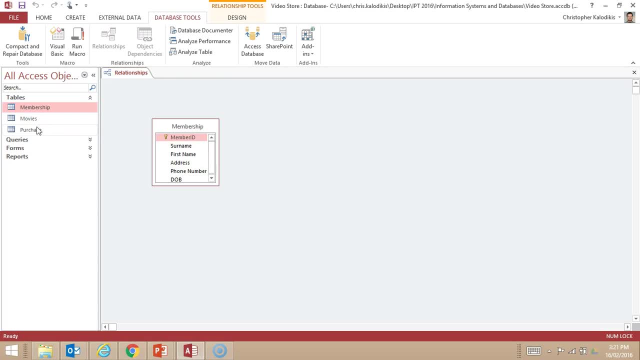 and I'm going to drag them on now. So I'm going to put on membership purchases in the middle, because it's going to be the one that's connecting everything- Okay, And movies, and now it's a piece of cake. all I've got to do is connect the primary key. 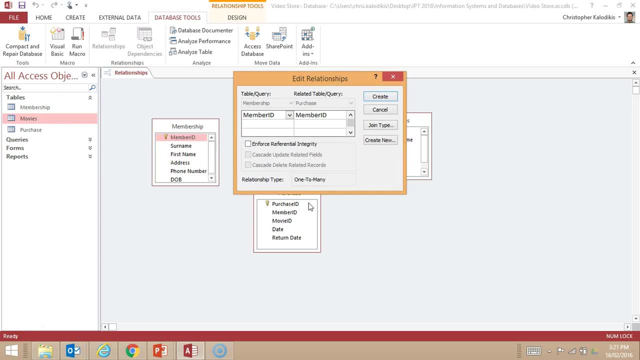 member ID to the foreign key member ID in the purchase database. It's made the connection and I'm going to enforce referral integrity create and it's established. it's a one to many connection. Then I'm going to do the same thing with movie ID to movie ID: its. 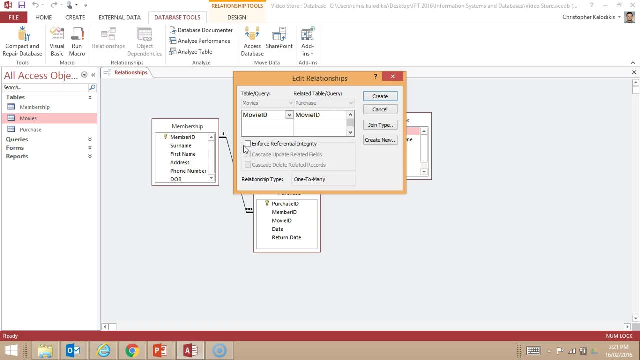 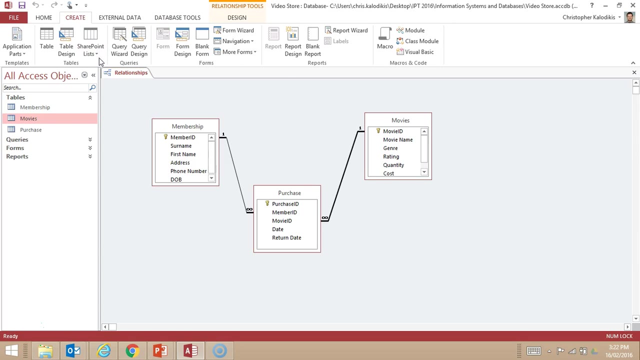 primary keys, foreign key, movie ID to movie ID enforcing integrity- and go Create Then. and i've now created my relational database. so now what i might do is test that it works. i'm going to do this by creating a query, so i'm going to go to create and i'm going to go query. i'll do it. 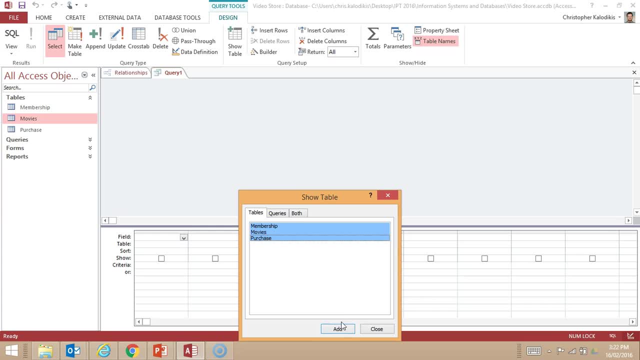 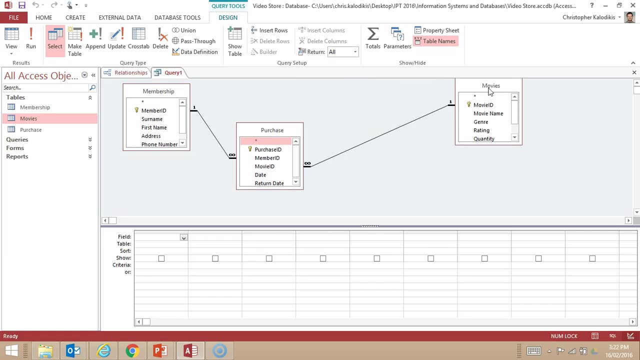 by design and i'm going to bring in all three databases, tables, and i might just make it so that purchases in the middle, and what i'll do is i'll do a check on what one of the users, based on on their id, has out rented at the moment. so, firstly, i'm going to put in the purchase id. 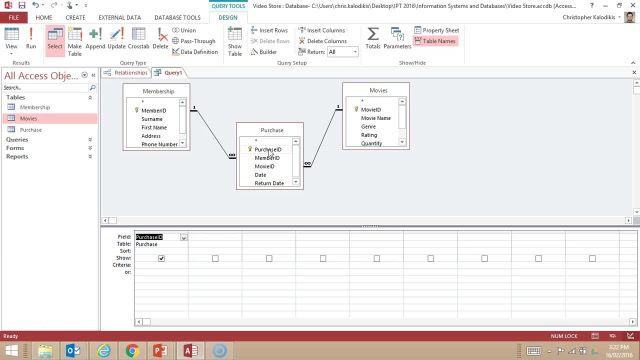 because i want to know under which purchase this transaction happened. i then want to know which member, based on their id, and i want to see their surname and first name attributes come up with this search as well. okay, i want to know what the member has specifically rented, so i need their movie id information and i want to know: 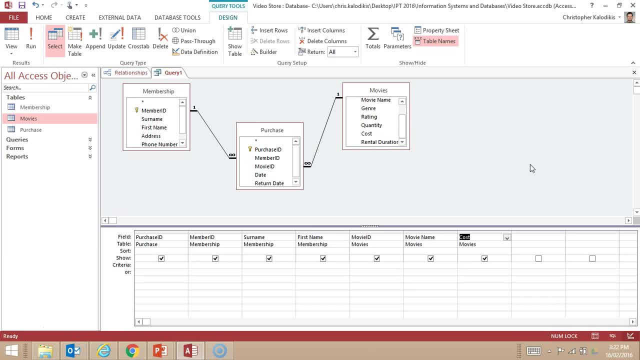 what movie it is and i want to know how much it costed. okay, and let's also see the rental duration. so i've basically got all three entities supplying different attributes to this search. now the only criteria i'm going to do in this search is i'm going to put in the members barcode, so this might. 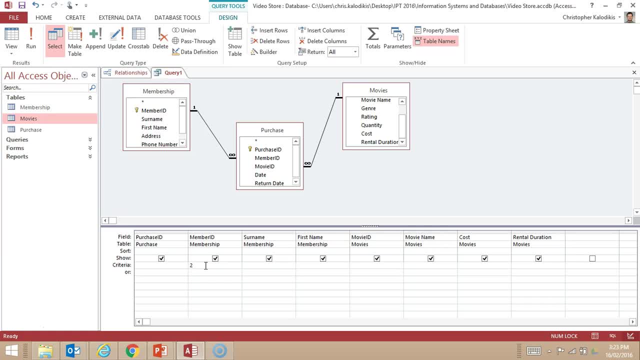 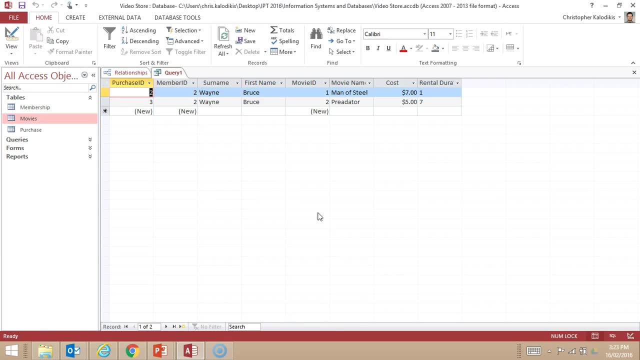 be when i scan their card. their card retrieves the number two. so whoever the member with the id 2 is, i want their information. i'm going to run this query and here it is: bruce wayne is the name of the member and they've rented two movies- it's man of steel and predator- and that is a cost of. 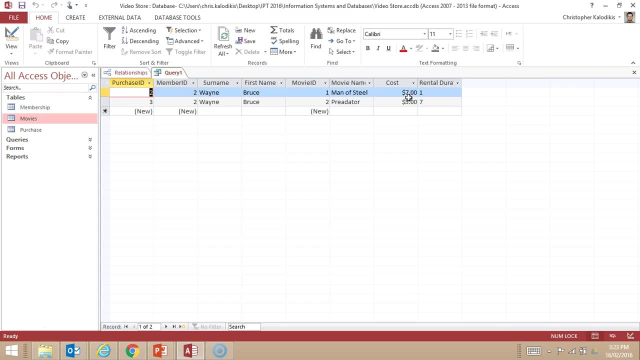 seven dollars and five dollars. so i can see that my relational database is actually working now because it brought in all these different attributes from the purchase id, from the actual membership id and from the actual movie id. i've got these fields, so three different entities, all supplied information, in one search. now i can also create: 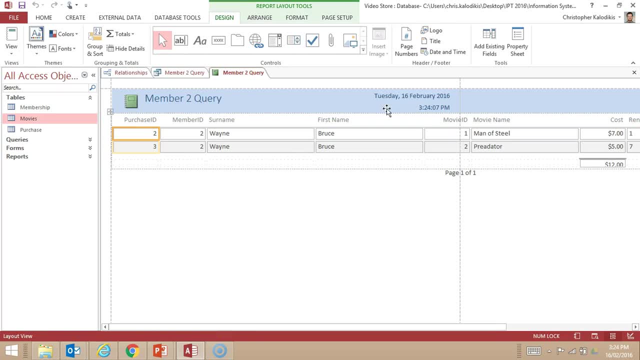 a report based on this information. now and now here's my database report and as you can see in the actual report, it actually gives me the total cost as well of this actual search. so can you see how making a relational database has actually made it quite interesting, that i can pull data.